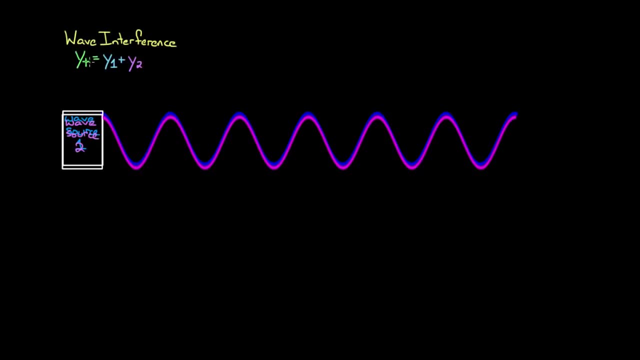 because wave interference happens when two waves overlap And if we wanna know what the total wave's gonna look like, we add up the contributions from each wave. So if I put a little backdrop in here and I add the contributions if the equilibrium point is right here. 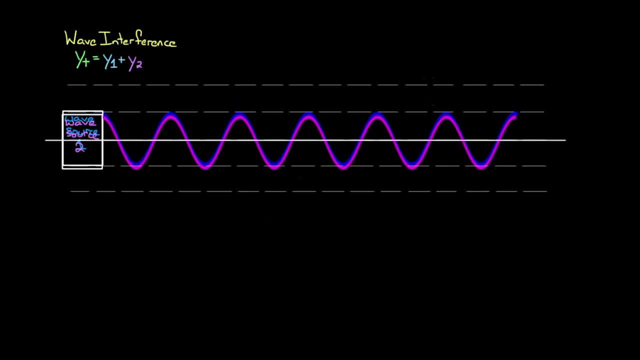 so that's where the wave would be zero. the total wave can be found by adding up the contributions from each wave. So if we add up the contributions from wave one and wave two, wave one here has a value of one unit. wave two has a value of one unit. 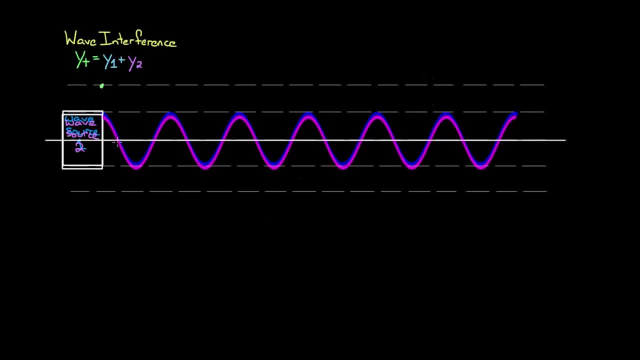 one unit plus one unit is two units, and then zero units, and zero units is still zero. Negative one and negative one is negative two, and you keep doing this and you realize, wait, you're just gonna get a really big cosine-looking wave. 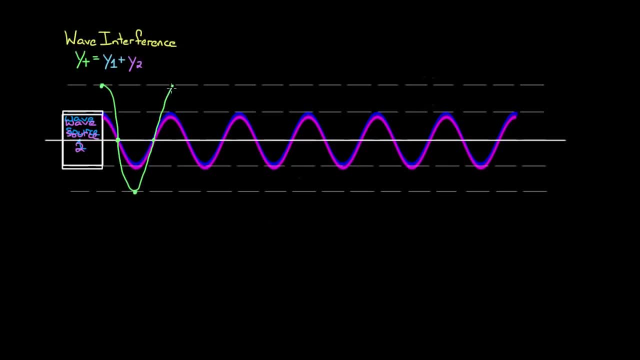 and it's gonna drop down to here And we say that these waves are constructively interfering. We call this constructive interference because the two waves combined to construct a wave that was twice as big as the original wave. So when two waves combine and form a wave, 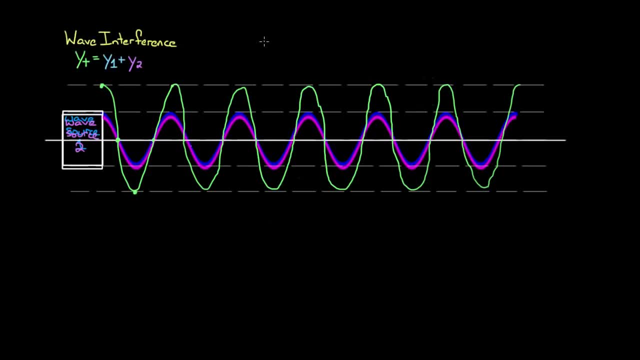 bigger than they were before. we call it constructive interference And because these two waves combined perfectly, sometimes you'll hear this as perfectly constructive or totally constructive interference. You can imagine cases where they don't line up exactly correct, but you still might get a bigger wave. 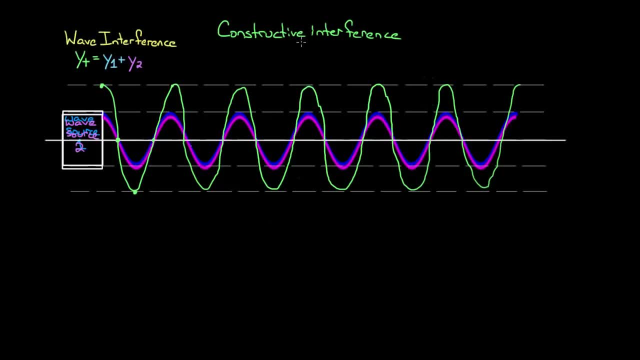 In that case it's still constructive. It might not be totally constructive, So that was constructive interference And these waves were constructive, think about it- because this wave source two looked exactly like wave source one did, and we just overlapped them. 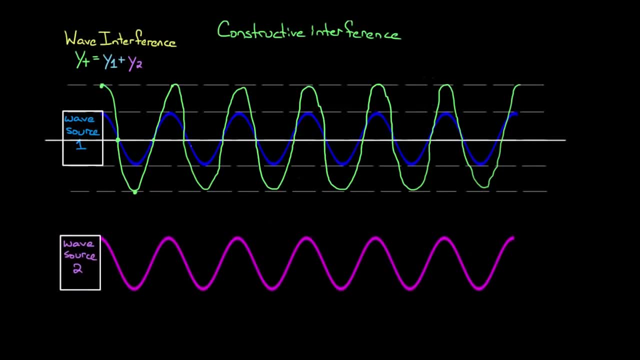 and we got double the wave, which is kinda like: all right, duh, that's not that impressive, But check this out. Let's say you had another wave source, a different wave source, two. This one is what we call pi shifted. 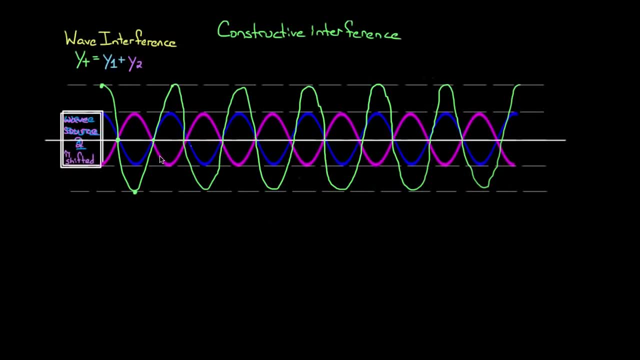 because, look at it, Instead of starting at a maximum, this one starts at a minimum compared to what wave source one is at. So it's one half of a cycle ahead of or behind of wave source one Half of a cycle is pi, because a whole cycle is two pi. 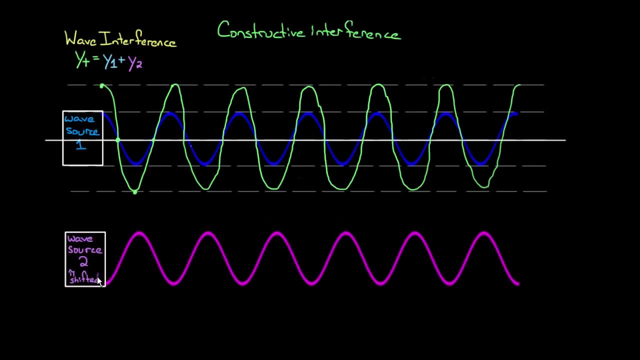 That's why people often call this pi shifted or 180 degrees shifted. Either way, it's out of phase from wave source one by half of a cycle. So what happens if we overlap these two? Now, I'm gonna take these two. 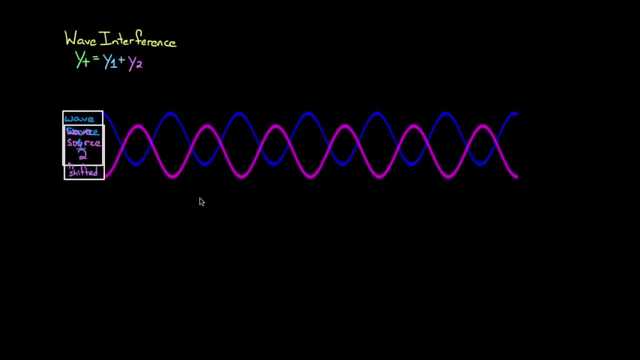 Let's get rid of that there. Let's just overlap these two and see what happens. I'm gonna overlap these two waves and we'll perform the same analysis. I don't really even need the backdrop now, because, look it, I've got one and negative one. 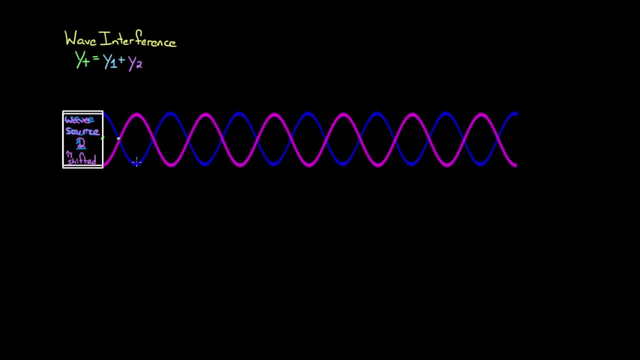 one and negative one. zero Zero and zero zero. Negative one and one zero, Zero and zero zero. No matter where I'm at, a half a negative, half zero, These two waves are gonna add up to zero. 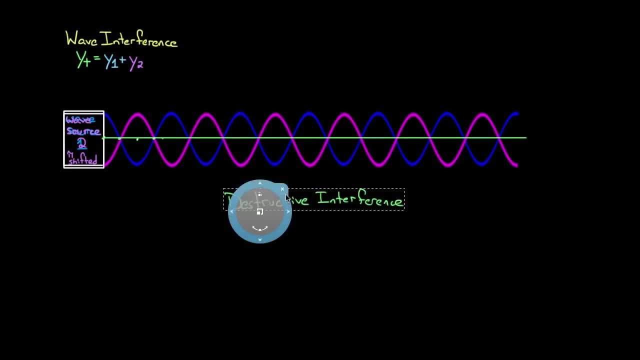 They add up to nothing. So we call this destructive interference, because these two waves essentially destroyed each other. This seems crazy: Two waves add up to nothing. How can that be the case? Are there any applications of this? Well, yeah, so imagine you're sitting on an airplane. 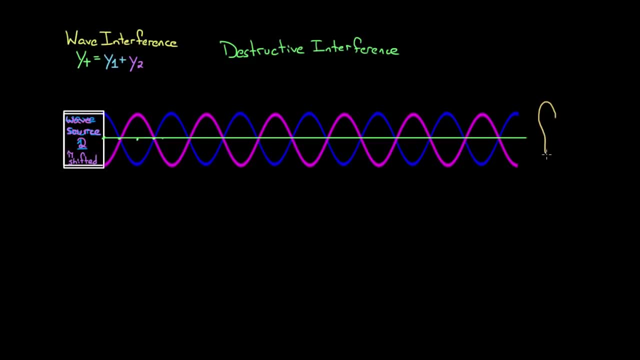 and you're listening to the annoying roar of the airplane engine in your ear. It's very loud and it might be annoying. So what do you do? You put on your noise-canceling headphones and what those noise-canceling headphones do. 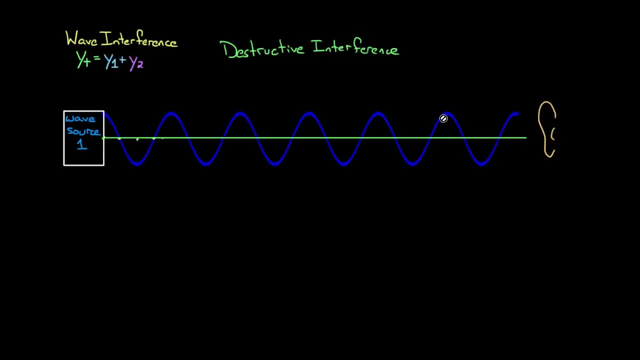 they sit on your ear. they listen to the wave coming in. This is what they listen to- this sound wave coming in- And they cancel off that sound by sending in their own sound, but those headphones pie-shift the sound that's going into your ear. 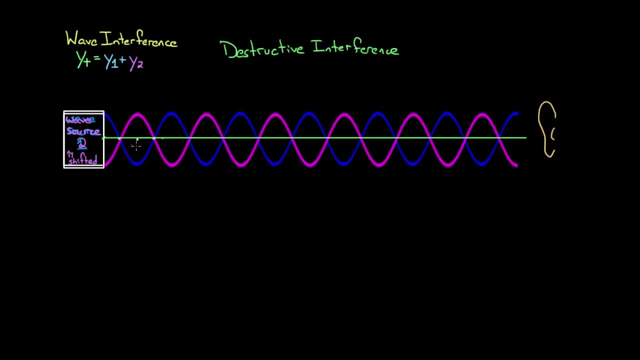 So they match that roar of the engine's frequency, but they send in a sound that's pie-shifted so that they cancel and your ear doesn't hear anything. Now, it's often not completely silent. they're not perfect, but they work surprisingly well. 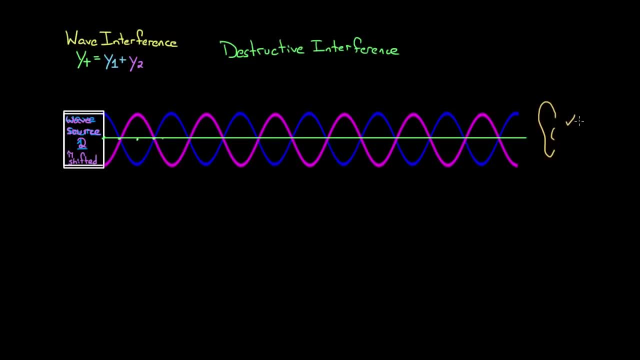 They're essentially fighting fire with fire. They're fighting sound with more sound and they rely on this idea of destructive interference. They're not perfectly, totally destructive, but the waves I've drawn here are totally destructive, If they were to perfectly cancel. 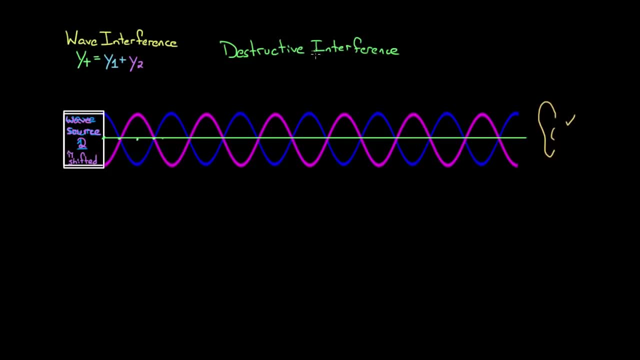 we'd call that total destructive interference or perfectly destructive interference. And it happens because this wave we sent in was pie-shifted compared to what the first wave was. So let me show you something interesting. If I get rid of all this, let me clean up this mess. 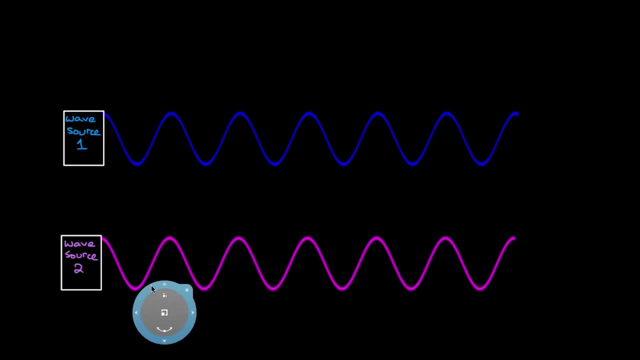 If I've got wave source one, let me get wave source two back. So this was the wave that was identical to wave source one. We overlap when we get constructive interference because the peaks are lining up perfectly with the peaks and these valleys or troughs are matching up perfectly. 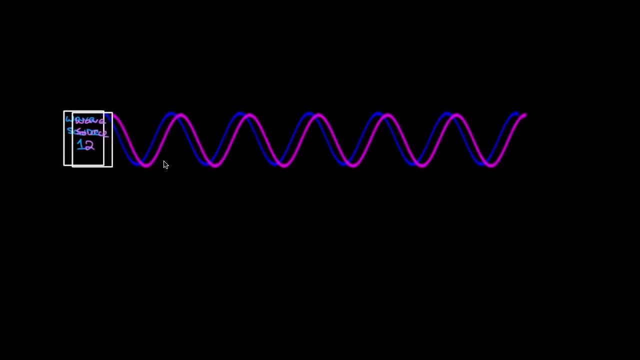 with the other valleys or troughs. But as I move this wave source two forward, look at what happens. They start getting out of phase. When they're perfectly lined up, we say they're in phase, they're starting to get out of phase. 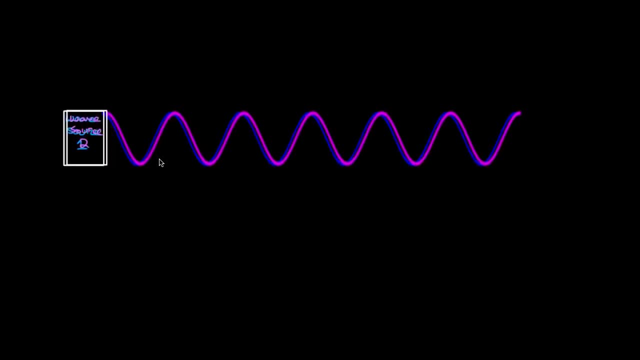 and look, when I move it forward enough, what was a constructive situation becomes destructive. Now all the peaks are lining up with the valleys. They would cancel each other out And if I move it forward a little more it lines up perfectly again and you get constructive. 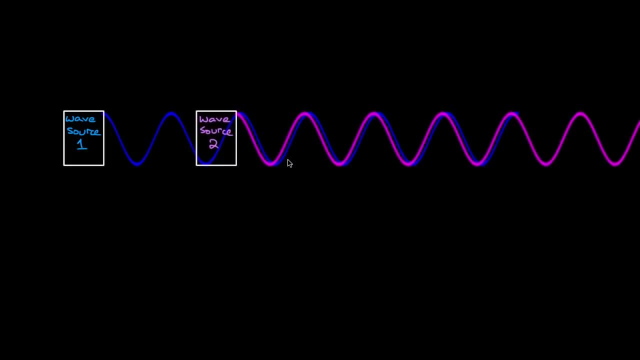 Move it more, I'm going to get destructive. Keep doing this. I go from constructive to destructive over and over. So, in other words, one way to get constructive interference is to take two wave sources that start in phase and just put them right next to each other. 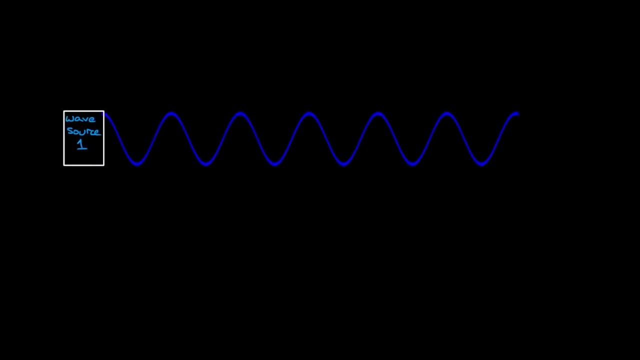 And a way to get destructive is to take two wave sources that are pi shifted out of phase and put them right next to each other and that'll give you destructive because all the peaks match the valleys. But another way to get constructive or destructive is to start with two waves that are in phase. 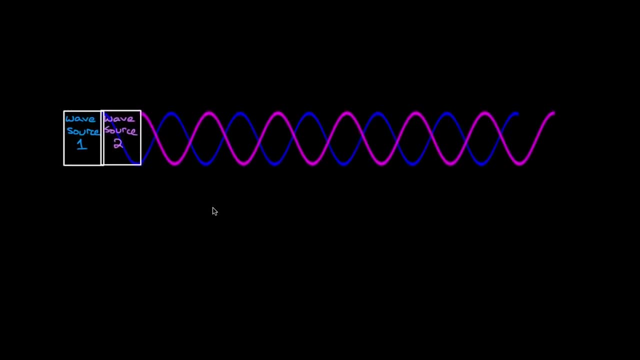 and make sure one wave is in phase and one wave gets moved forward compared to the other. But how far forward should we move these in order to get constructive and destructive? Well, let's just test it out. We start here. When they're right next to each other, we get constructive. 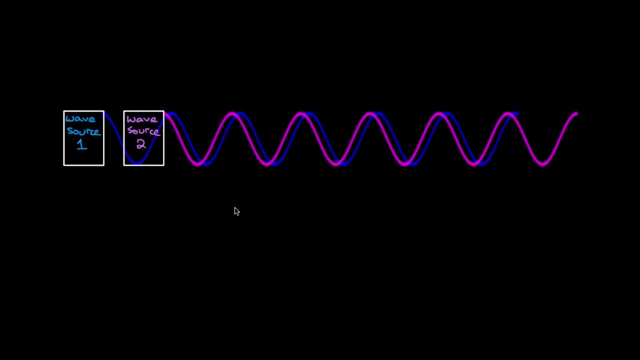 And if I move this second wave source that was initially in phase all the way to here, I get constructive again. How far did I move it? I moved it this far. The front of that speaker moved this far. So how far was that? 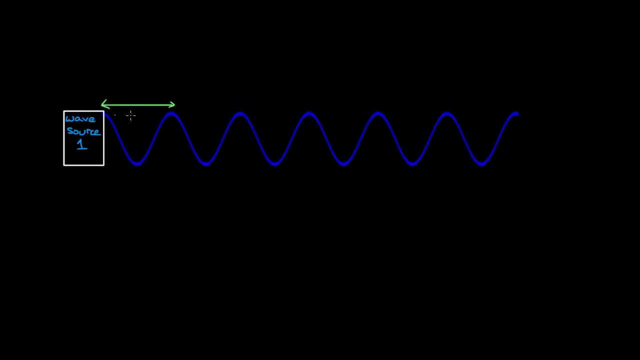 Let me get rid of this. That was one wavelength, So look at this picture. From peak to peak is exactly one wavelength. We're assuming these waves have the same wavelength. So notice that essentially what we did. we made it so that the wave from wave source two 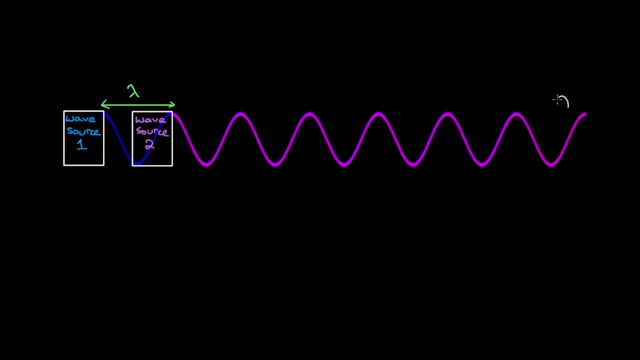 doesn't have to travel as far to whatever's detecting the sound. Maybe there's an ear here or some sort of scientific detector detecting the sound. Wave source two is now only traveling this far to get to the detector, whereas wave source one is traveling this far. 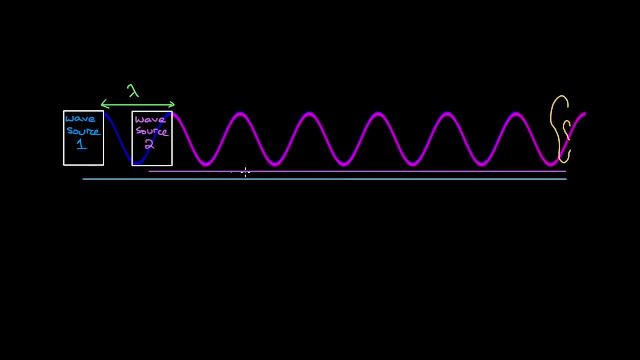 In other words, we made it so that wave source one has to travel one wavelength further than wave source two does, and that makes it so that they're in phase and you get constructive interference again. But that's not the only option. We can keep moving wave source two forward. 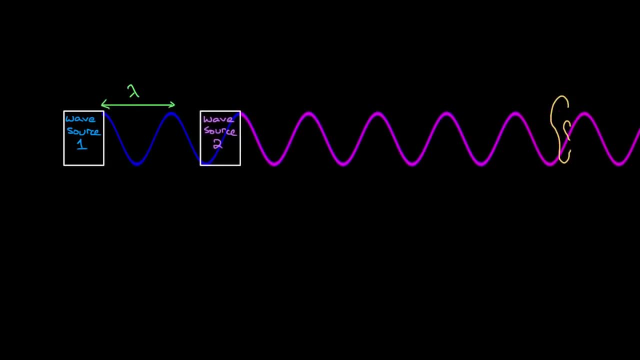 If we move it all the way to here, we've moved it another wavelength forward. We again get constructive interference, And at this point wave source one is having to make its wave travel two wavelengths further than wave source two does, And you can probably see the pattern. 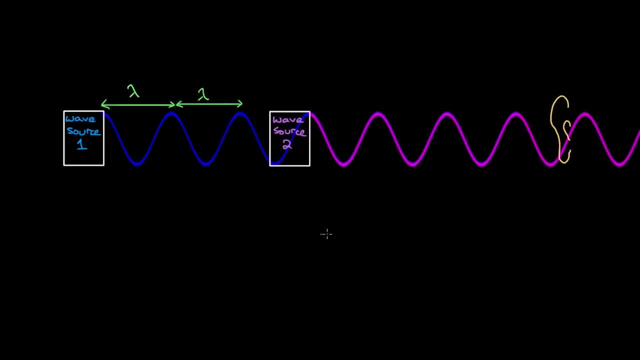 No matter how many wavelengths we move it forward, as long as it's an integer number of wavelengths, we again get constructive interference. So something that turns out to be useful is a formula that tells us: all right, how much path length difference should there be? 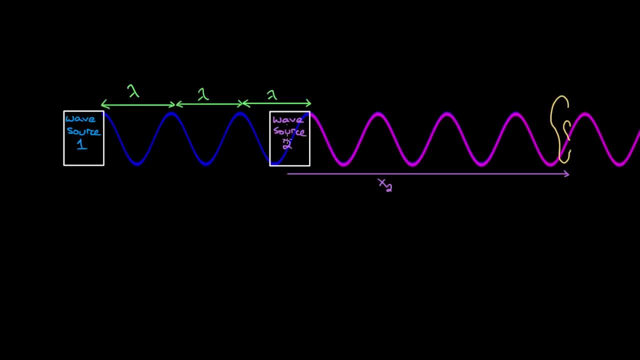 So if I'm going to call this x2, the distance that the wave from wave source two has to travel to get to whatever's detecting that wave, and the distance x1 that wave source one has to travel to get to that detector. So we could write down a formula. 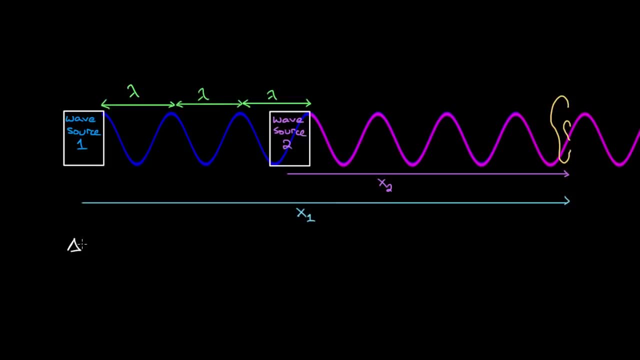 that relates the difference in path length. I'll call that delta x, which is going to be the distance that wave one has to travel, minus the distance that wave two has to travel. and, given what we saw up here, if this path length difference is ever equal to, 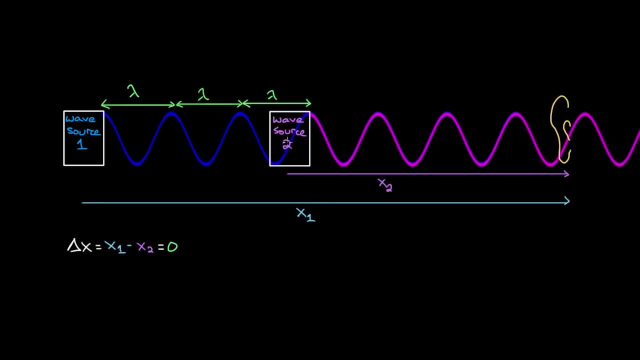 an integer number of wavelengths. so if it was zero, that was when they were right next to each other- you got constructive. When this difference is equal to one wavelength, we also got constructive. When it was two wavelengths, we got constructive. 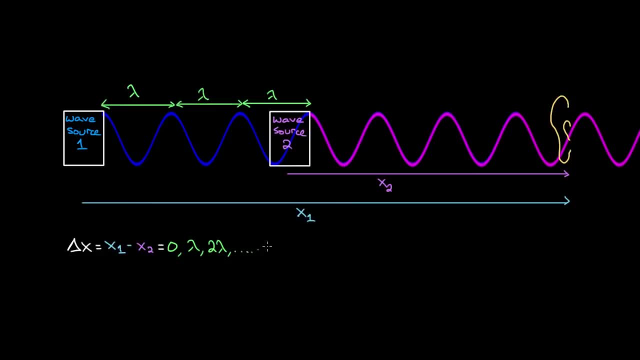 It turns out, any integer wavelength gives us constructive. So how would we get destructive interference then? Well, let's continue with this wave source that originally started in phase right. So these two wave sources are starting in phase. How far do I have to move it to get destructive? 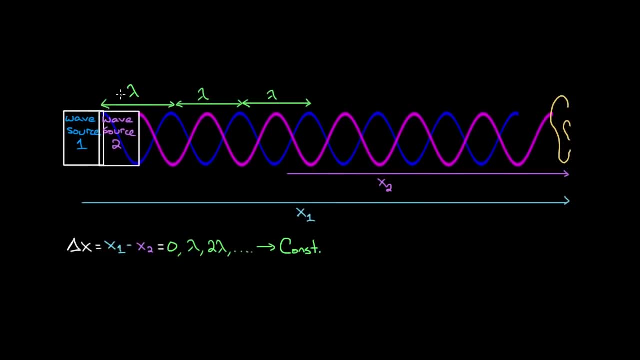 Let's just see I have to move it till it's right about here. So how far did the front of that speaker move? It moved about this far which, if I get rid of that speaker, you could see is about half of a wavelength. 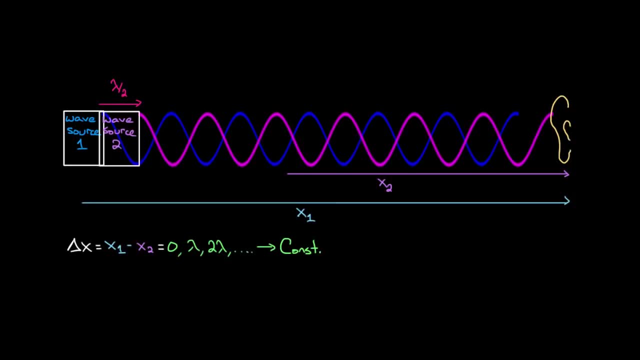 From peak to valley is one half of a wavelength, But that's not the only option. I can keep moving it forward. Let's just see That's constructive. My next destructive happens here. which was an extra this far. How far was that? 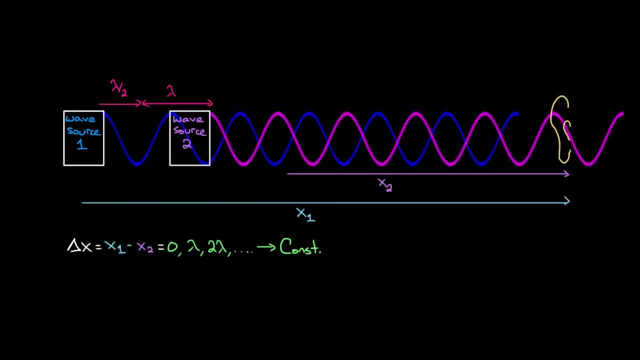 Let's just see That's one wavelength. So notice, at this point wave source one is having to go one and a half wavelengths further than wave source two does. So let's just keep going. Move wave source two. That's constructive. 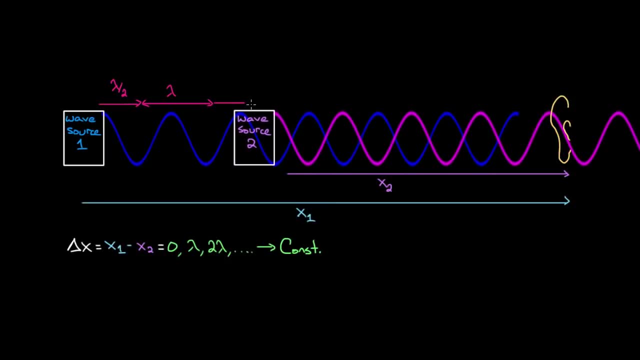 We get another destructive here which is an extra this far forward, And that's equal to one more wavelength. So if we get rid of this, you could see valley to valley is a whole another wavelength. So in this case, wave source two has to travel. 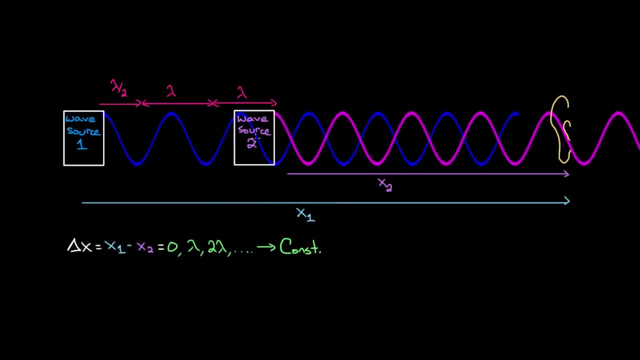 two and a half wavelengths, Two and a half wavelengths farther than wave source two. Anytime wave source one has to travel a half integer more wavelengths than wave source two, you get destructive interference. In other words, if this path length difference here is equal to lambda over two, 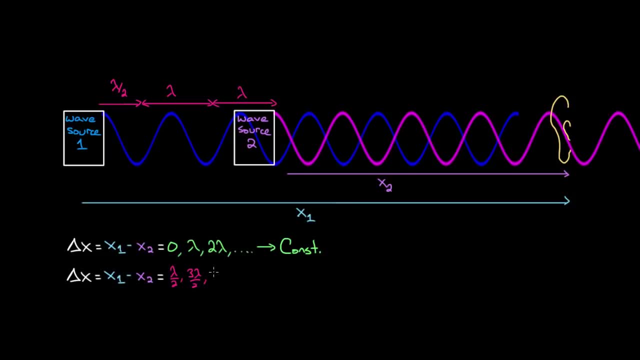 three lambda over two, which is one and a half wavelengths, five lambda over two, which is two and a half wavelengths, and so on. that leads to destructive interference. So this is how the path length differences between two wave sources can determine whether you're gonna get constructive. 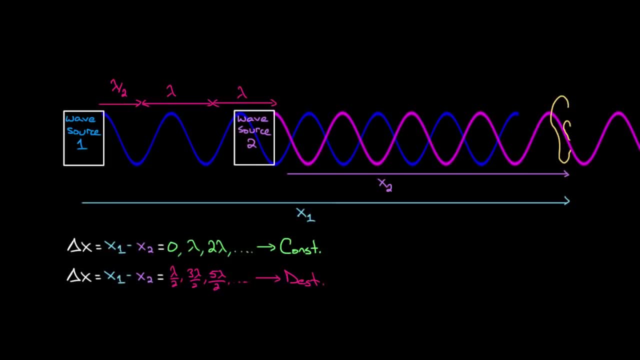 or destructive interference. But notice, we started with two wave sources that were in phase. These started in phase. So this whole analysis down here assumes that the two sources started in phase with each other, ie neither of them are pi shifted. 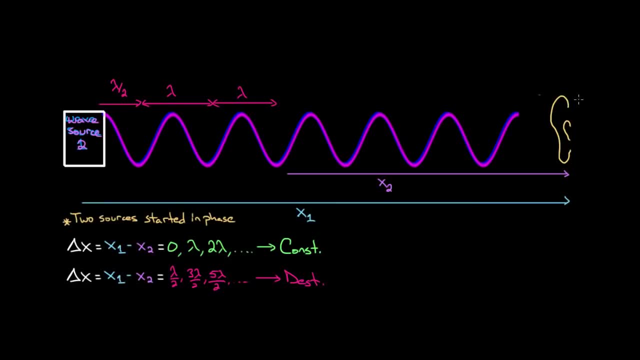 What would this analysis give you if we started with one that was pi shifted? So let's get rid of this wave two. Let's put this wave two back in here. Remember this one. This one was pi shifted. Pi shifted relative to wave source one. 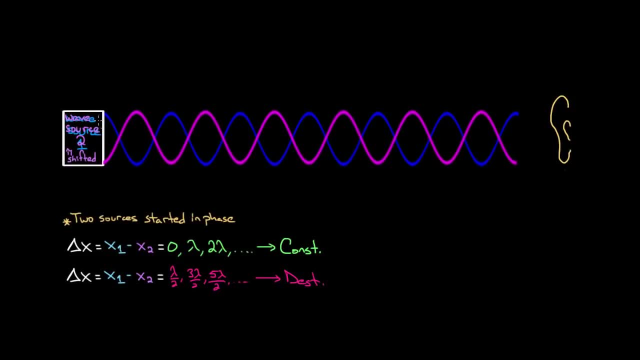 So we'll put this one in here and we'll get rid of this. Now, when these two wave sources are right next to each other, you're getting destructive interference. So this time, for a path length difference of zero, these are both traveling the same distance. 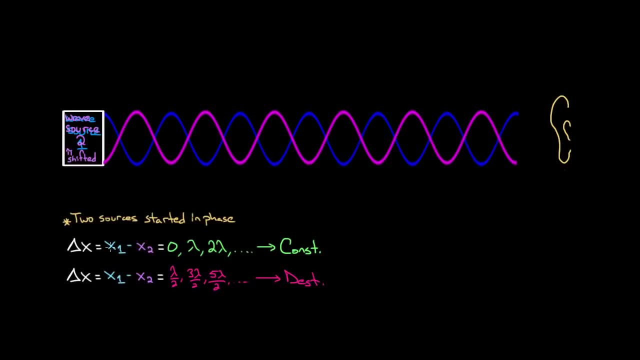 to get to the detector. So x one and x two are gonna be equal. You subtract them, you'd get zero. This time the zero's giving us destructive instead of constructive. So let's see what happens If we move this forward. 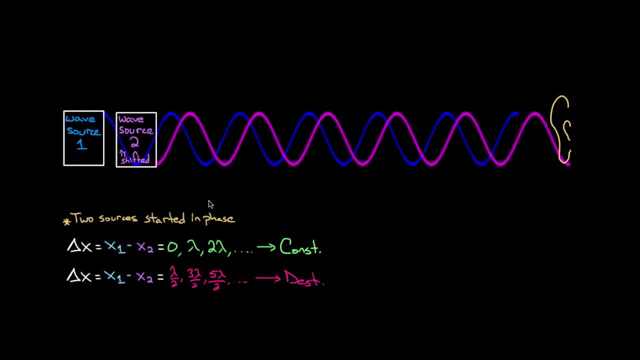 let's see how far we've gotta move this forward. to again get destructive, We'd have to move it over to here. How far did we move it? Let's just check. We moved the front of this speaker that far, which is one whole wavelength. 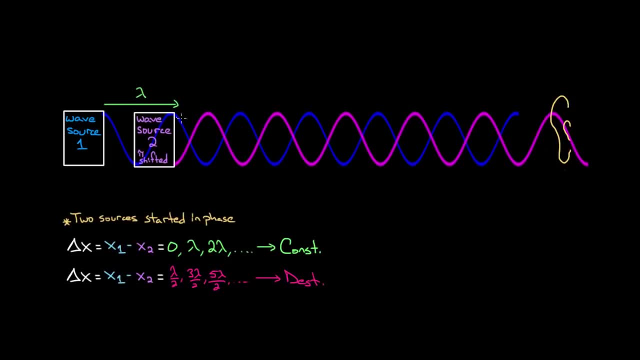 So if we get rid of this, we had to move the front of the speaker one whole wavelength and look it again, it's destructive. So again, zero gave us destructive this time, and lambda's giving us destructive, and you realize. 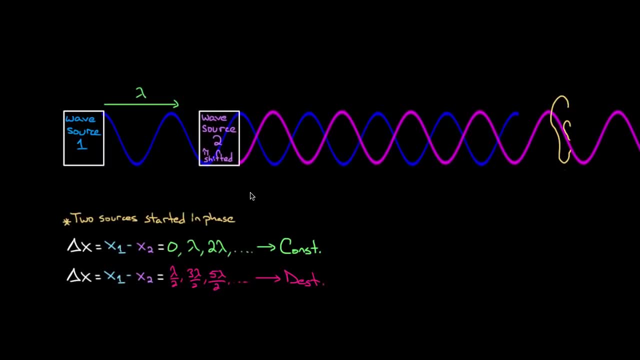 oh wait, all of these integer wavelengths. if I move it another integer wavelength forward, I'm again gonna get destructive interference, because all these peaks are lining up with it, All these valleys. So, interestingly, if two sources started pi out of phase. 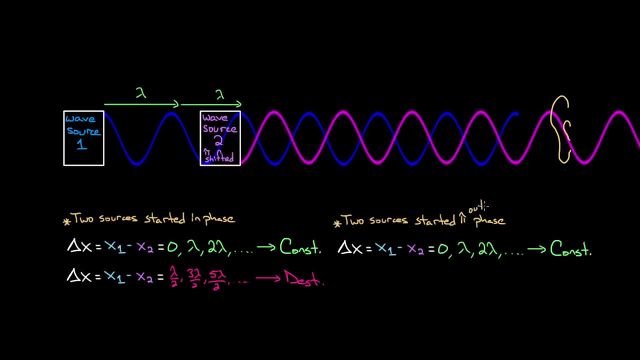 so I'm gonna change this. started pi out of phase then path length differences of zero lambda and two lambda aren't gonna give us constructive, they're gonna give us destructive. And so you could probably guess now what are these path length differences? 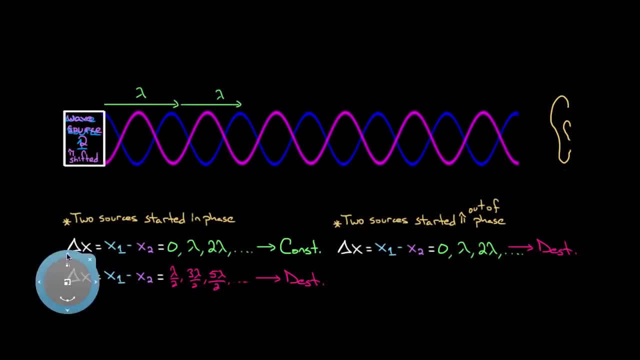 of half integer wavelengths gonna give us. Well, let's just find out, Let's start here and we'll get rid of these. Let's just check, We'll move this forward one half of a wavelength and what do I get? Yep, I get constructive. 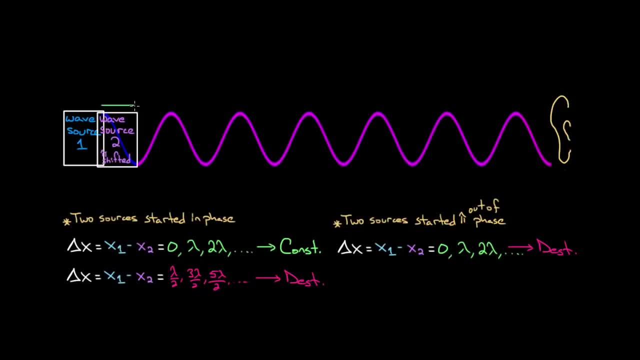 So if I move this pi shifted source half a wavelength forward, instead of giving me destructive, it's giving me constructive now. And if I move it so it goes another wavelength forward over to here. notice, this time wave source one has to move one and a half wavelengths. 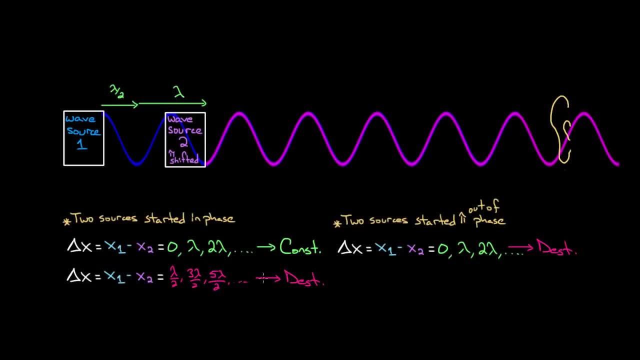 further than wave source two, that's three halves wavelengths. But instead of giving us destructive- look, these are lining up perfectly- it's giving us constructive. and you realize, oh, all these half integer wavelength, path length differences, instead of giving me destructive, 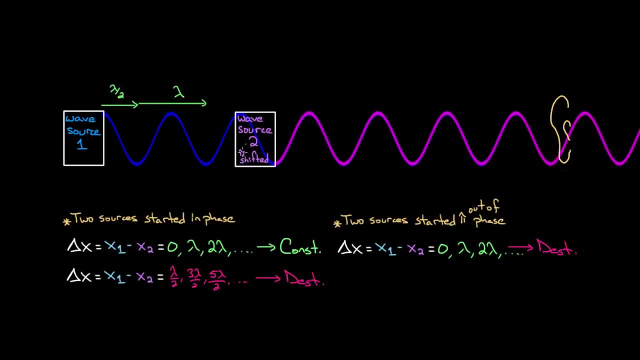 are giving me constructive now, because one of these wave sources was pi shifted compared to the other. So I can take this here and I can say that when the two sources start pi out of phase, instead of leading to destructive, this is gonna lead to constructive interference. 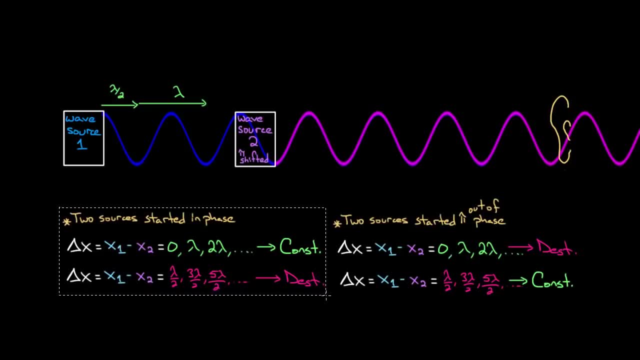 And these two ideas are the foundation of almost all interference patterns you find in the universe, which is kind of cool. If there's an interference pattern you see out there, it's probably due to this, And if there's an equation, you end up using. 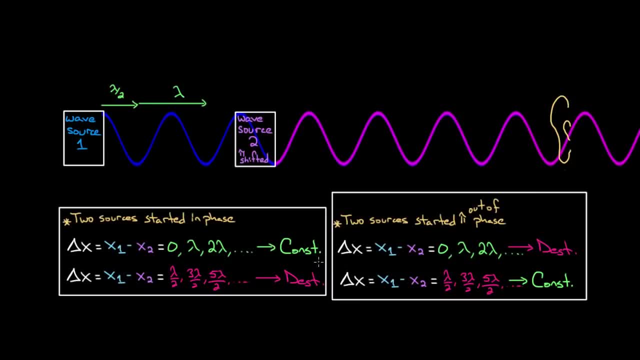 it's probably fundamentally based on this idea if it's got wave interference in it. So I should say one more thing: that sources don't actually have to start out of phase. Sometimes they travel around, things happen. it's a crazy universe. 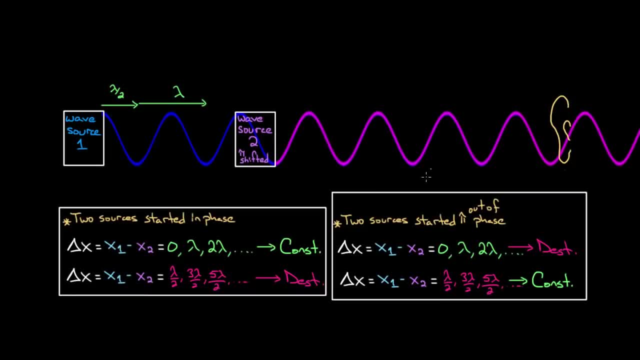 Maybe one of the waves gets shifted along its travel. Regardless, if any of them get a pi shift, either at the beginning or later on, you would use this second condition over here to figure out whether you get constructive or destructive If neither of them get a phase shift. 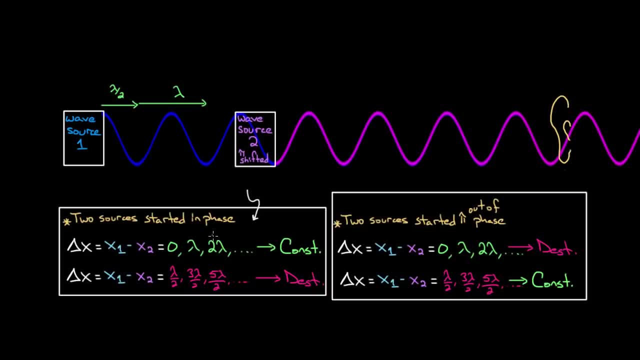 or, interestingly, if both of them get a phase shift, you could use this one, because you could imagine flipping both of them over and it's the same as not flipping any of them over. So recapping constructive interference happens when two waves are lined up perfectly.